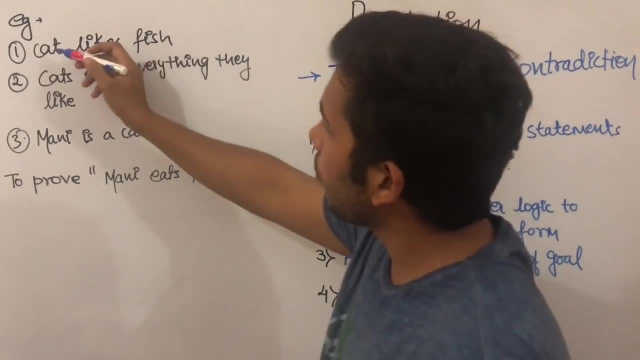 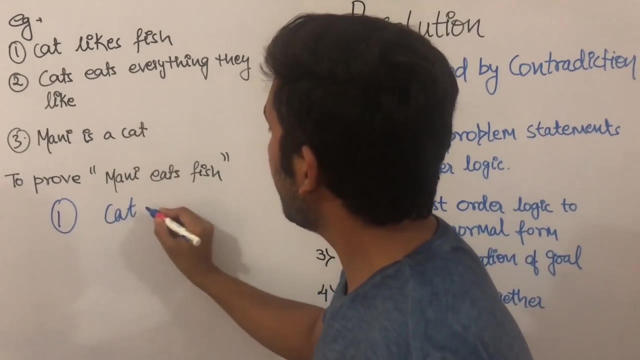 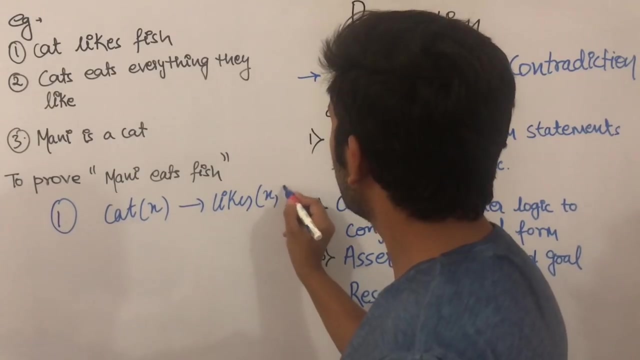 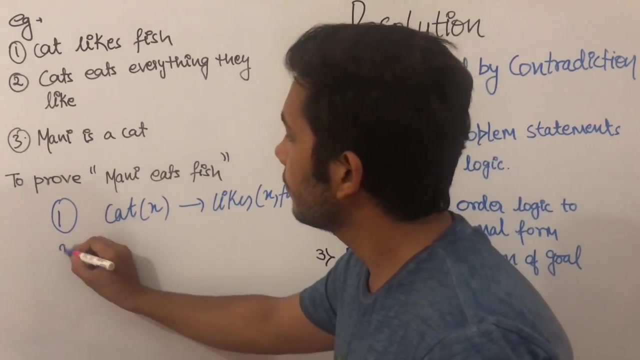 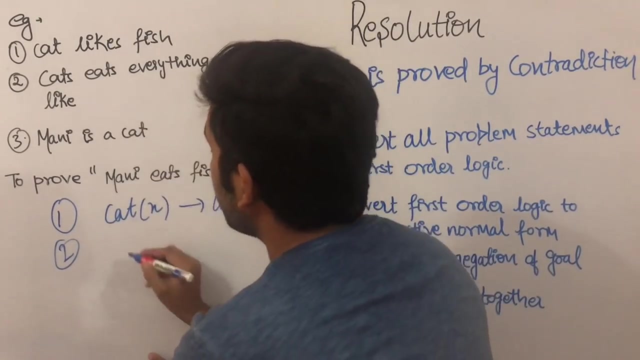 have to convert the statement into first order logic. then what is the first order logic of this? cat likes fish. you can write cat likes fish. it is the predicate logic of the given statement. now the second cat eats everything they like. so for this statement you can write it as cat. 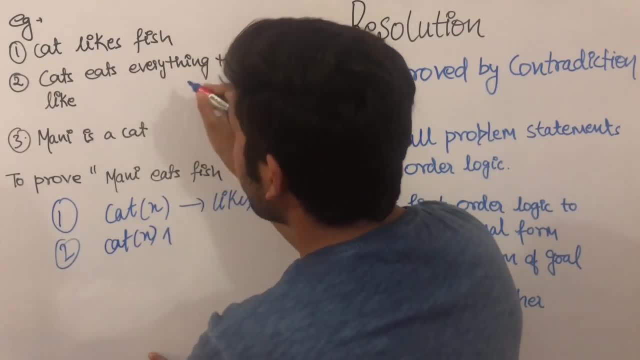 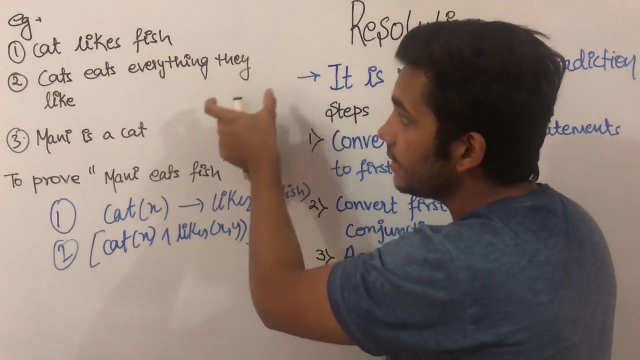 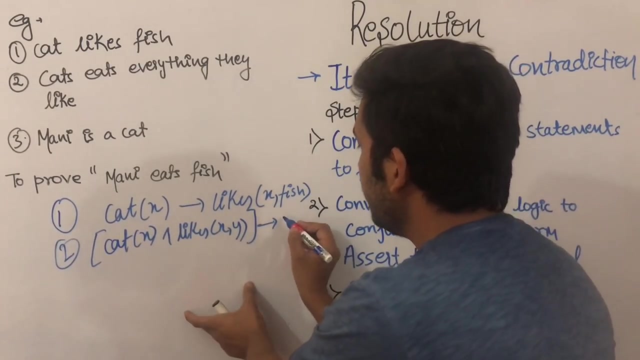 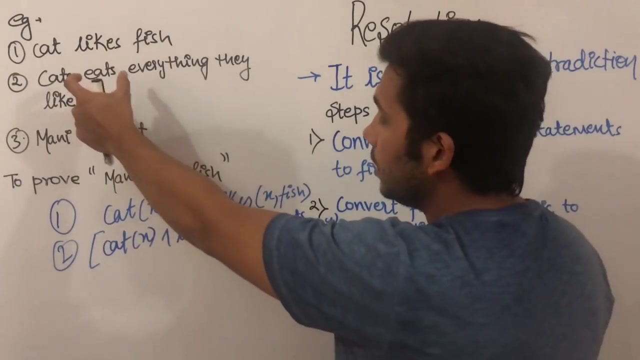 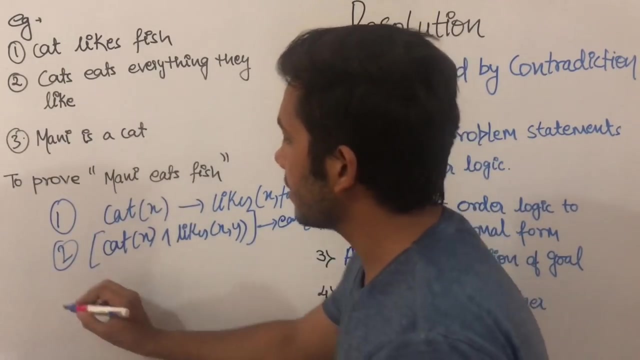 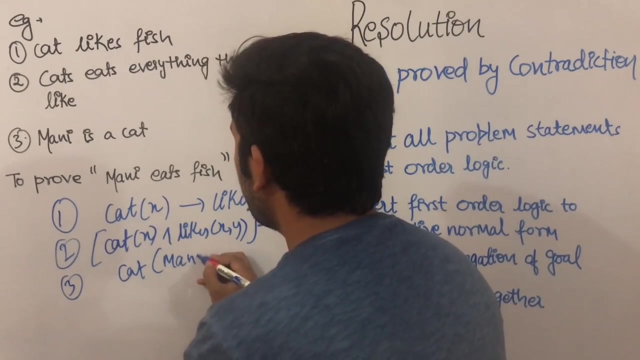 likes fish and likes X comma Y. so whatever cat likes they eat. so you can write cat and likes. so whatever cat likes she eats, X comma Y. so this was the predicate logic of the second statement. now coming to the third statement, that is, money is a cat, so you can write it directly as cat money. now we have to prove money eat. 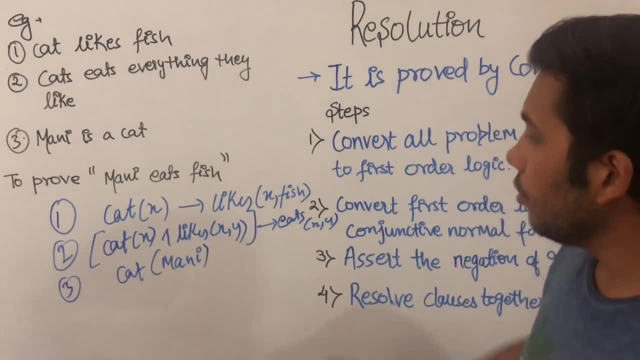 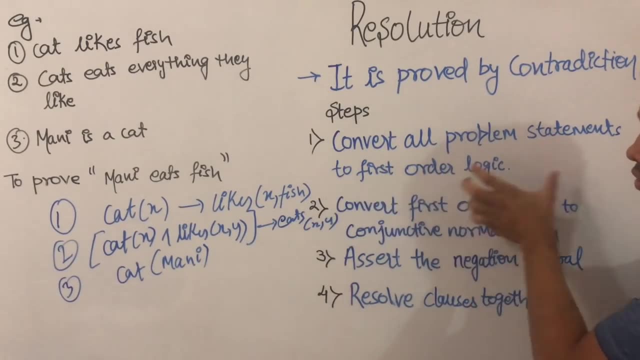 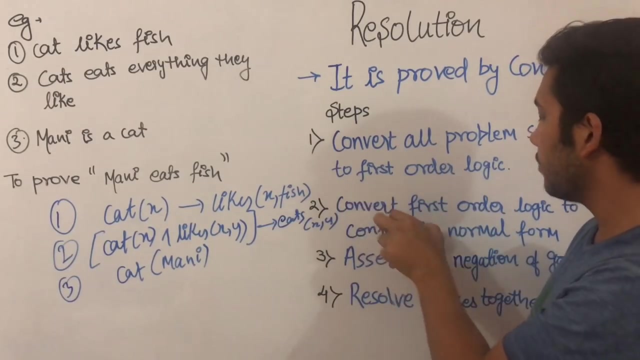 eats fish. so for this statement, first, in the first step, we have converted the given statement into first order logic. now the second step: we will convert this first order logic statement into conjunctive normal form. so so in my previous video I tell about the rules to convert the predicate logic. 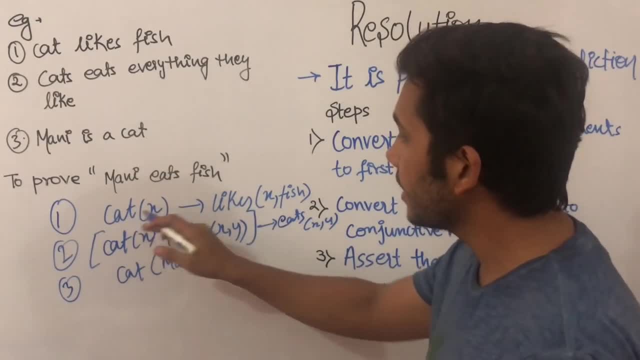 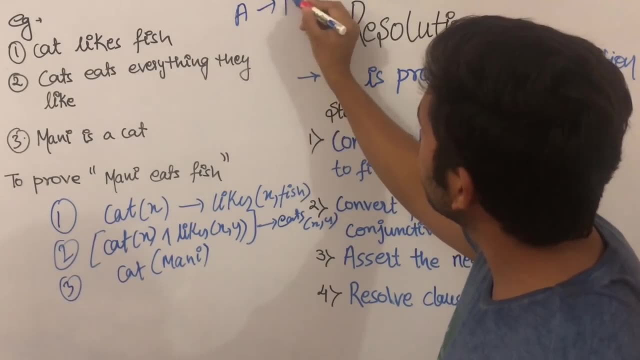 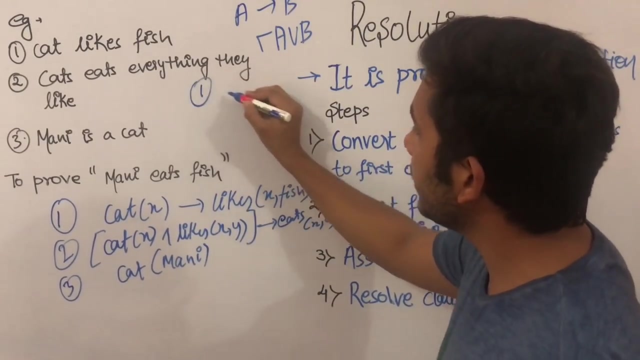 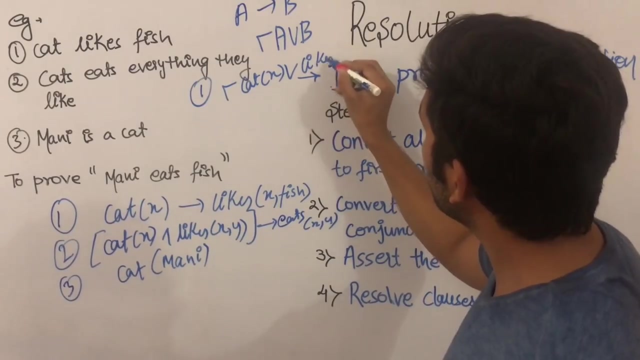 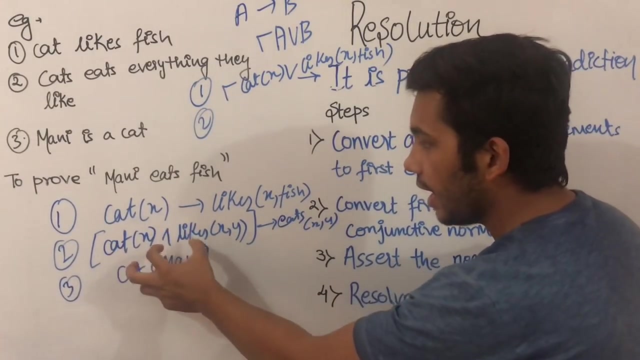 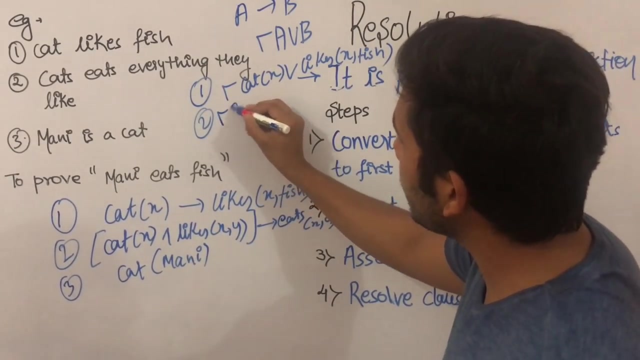 into a conjunctive normal form for this statement: cats like fish. you can say: as a implies b, this can be written as negotiation of a or b. so this statement can be written as negotiation of cat x or likes x comma fish. in second statement: cat and likes x comma y, each fish. so this is a and this is b. this can be written as negotiation of. 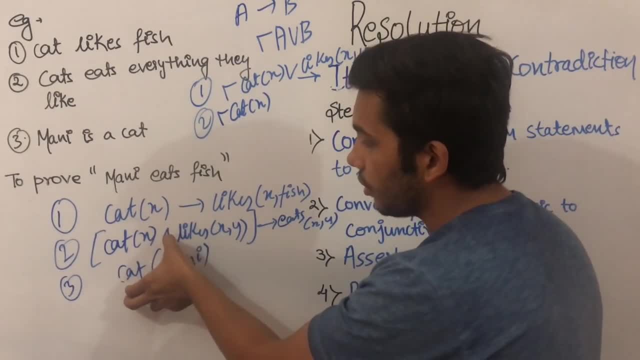 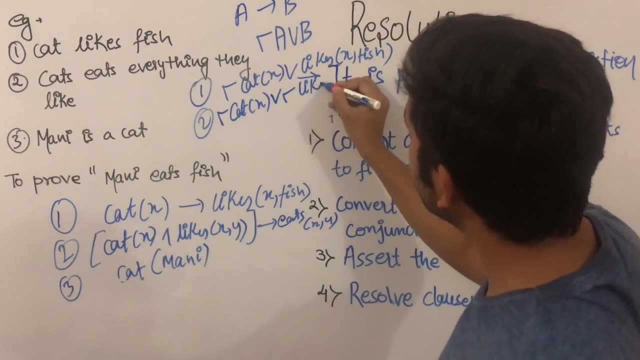 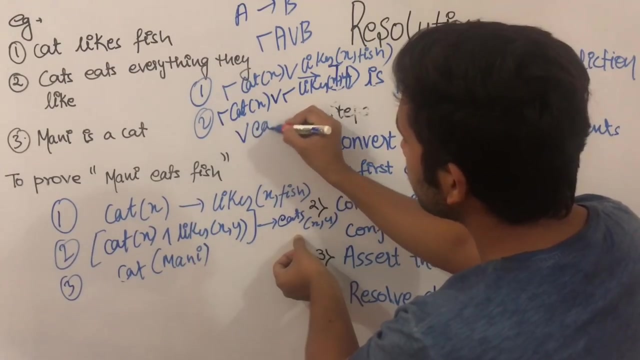 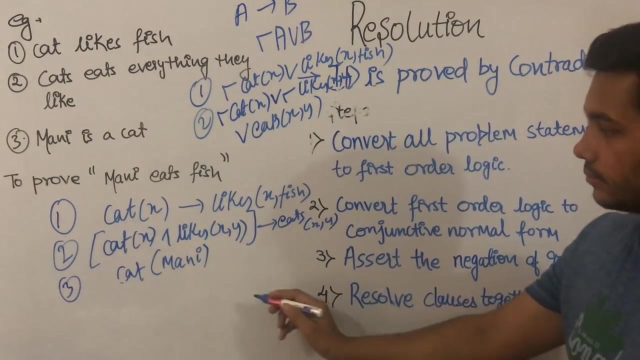 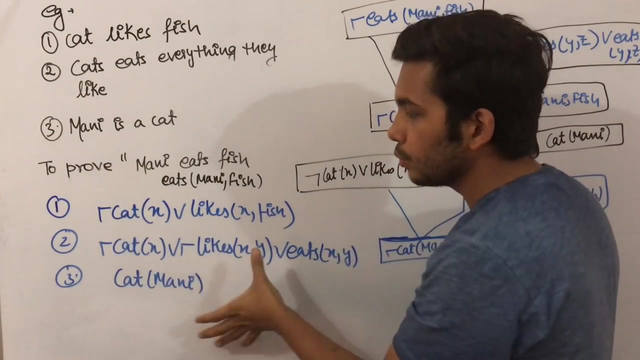 cat x and negotiation in front of and convert into or, so you can write it as: or. negotiation likes x comma y and this finally converts into eats: x comma y. and this statement b we write as it is. so this was our example and after converting from predicate logic to cnf form, 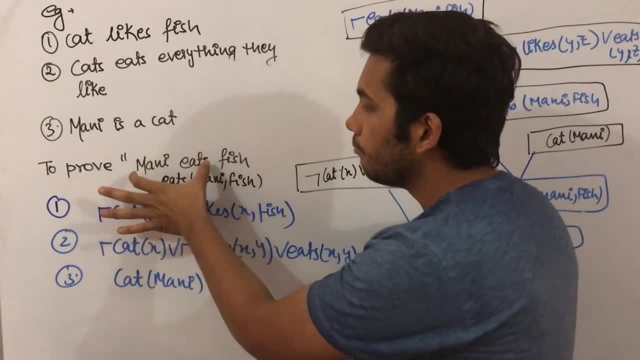 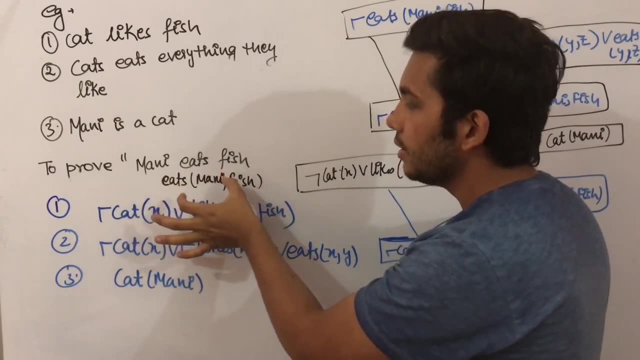 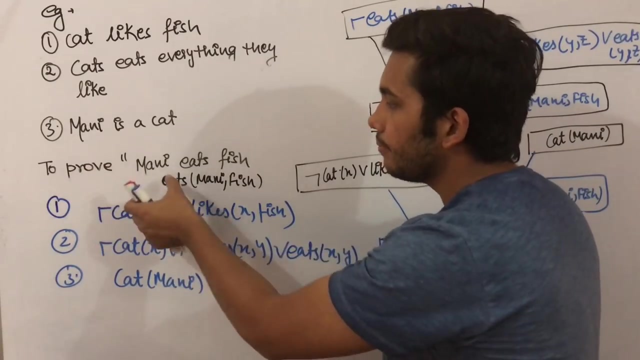 this was our statement and we need to prove money eats fish so we can write this statement as eats money, comma fish. so in resolution we prove by contradiction. so if we need to prove this money eats fish, then we can write as it is. so we can write as it is. so we can write as it is. 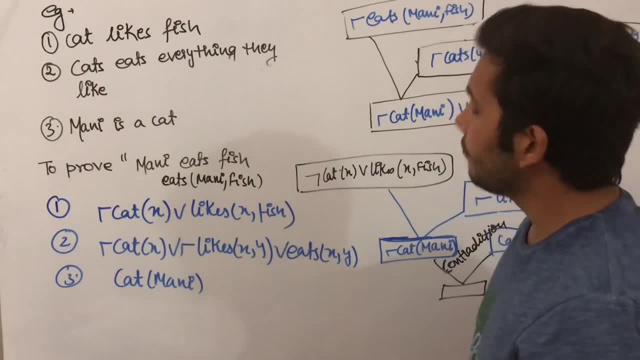 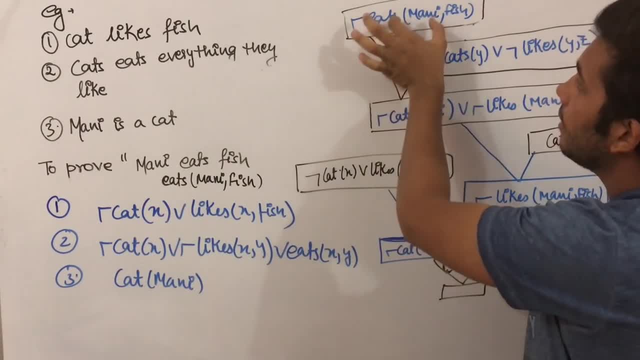 comma fish. so we have considered this statement. negotiation of negotiation of eats money. negotiation of negotiation of eats money. negotiation of negotiation of eats money, comma fish. we want to prove its money, comma fish. we want to prove its money, comma fish. we want to prove its money, comma fish. so we have taken negotiation of: 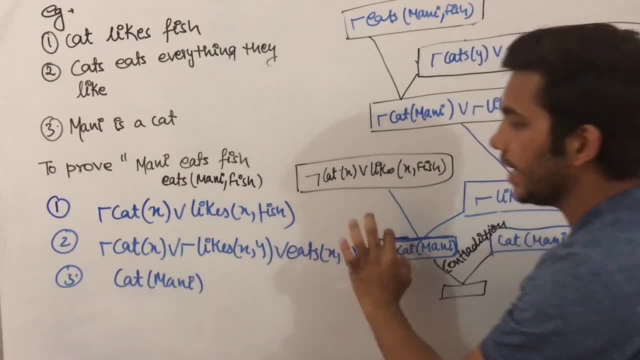 comma fish. so we have taken negotiation of comma fish. so we have taken negotiation of its money comma fish. so from second its money comma fish. so from second its money comma fish. so from second statement we can pick any statement at statement. we can pick any statement at: 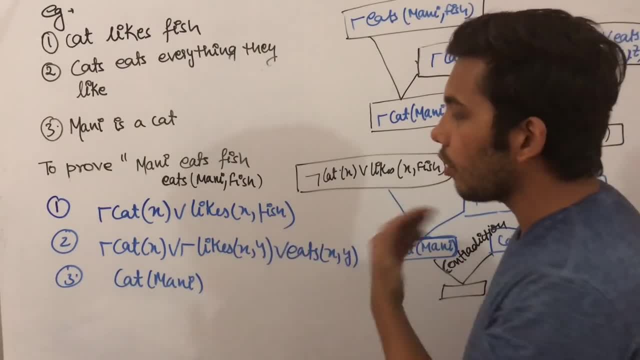 statement. we can pick any statement at any time because how we are going to cut any time, because how we are going to cut any time, because how we are going to cut or dissolve the part negotiation part or dissolve the part negotiation part or dissolve the part negotiation part, like in this: eats, money, comma, fish and 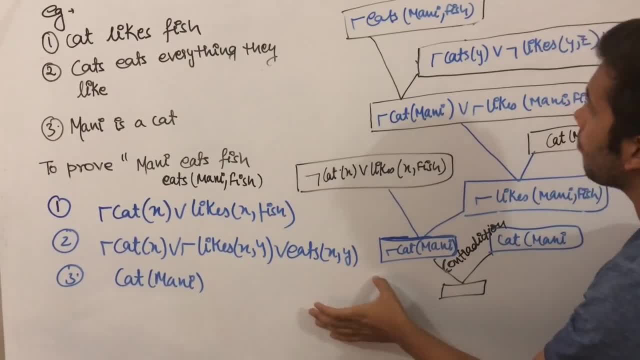 like in this eats money comma fish, and like in this eats money comma fish and in this in second statement we have each in this in second statement, we have each in this in second statement. we have each X comma Y, so on negotiation part, and a X comma Y, so on negotiation part and a. 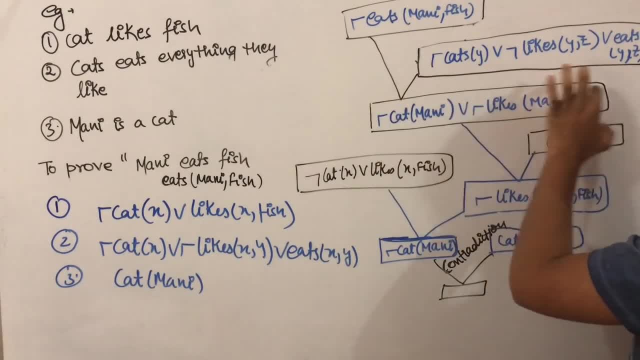 X comma Y, so on. negotiation part and a non-negotiated part will get cancel, each non-negotiated part will get cancel. each non-negotiated part will get cancel each other and we will get the result so this other and we will get the result so this. 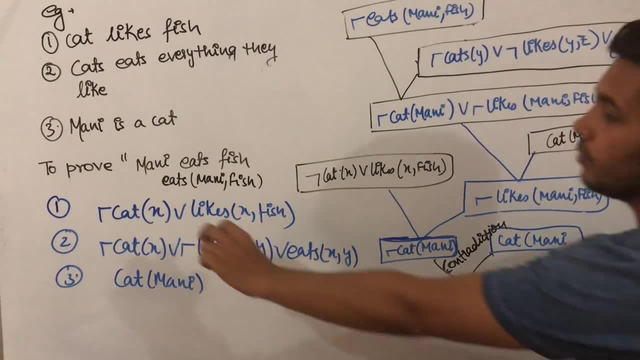 other and we will get the result. so this was our statement: eats money, comma fish was our statement. eats money, comma fish was our statement. eats money, comma fish. and from second statement we have and from second statement we have and from second statement we have negotiation of cat Y or likes Y, comma Z. 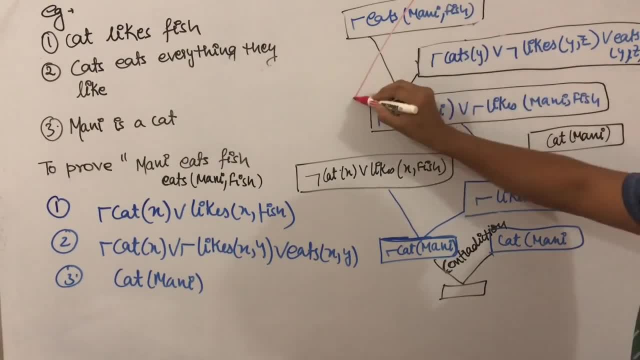 negotiation of cat Y or likes Y comma Z. negotiation of cat Y or likes Y comma Z. eats Y comma Z. so now we can cancel this. eats Y, comma Z. so now we can cancel this. eats Y comma Z. so now we can cancel this statement. and this statement because this: 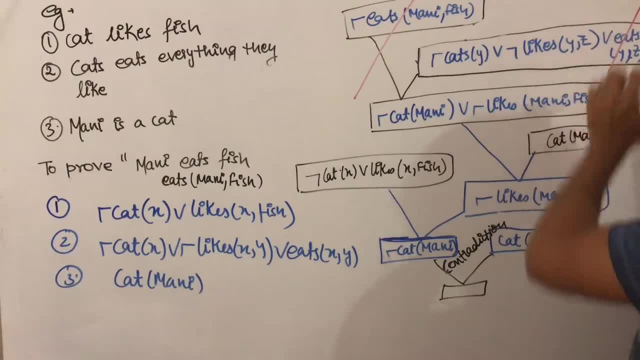 statement and this statement, because this statement and this statement, because this is a negotiation part and this is a is a negotiation part, and this is a is a negotiation part, and this is a positive part. so positive, negative get positive part. so positive, negative, get positive part. so positive, negative get cancelled. now, after cancelling the, 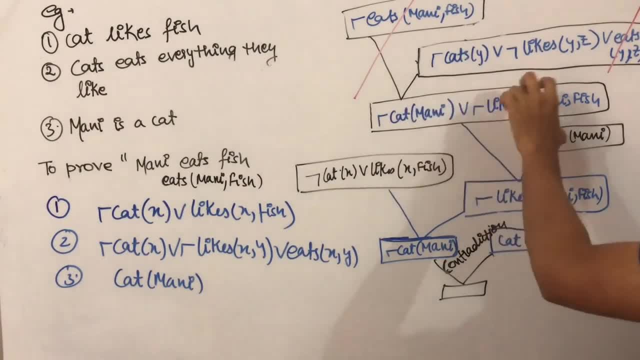 cancelled. now, after cancelling the cancelled now, after cancelling the negotiation parts, what is the remaining negotiation parts? what is the remaining negotiation parts? what is the remaining item? we have negotiation of cat. you can item. we have negotiation of cat, you can item. we have negotiation of cat, you can. in place of why you can put the value. 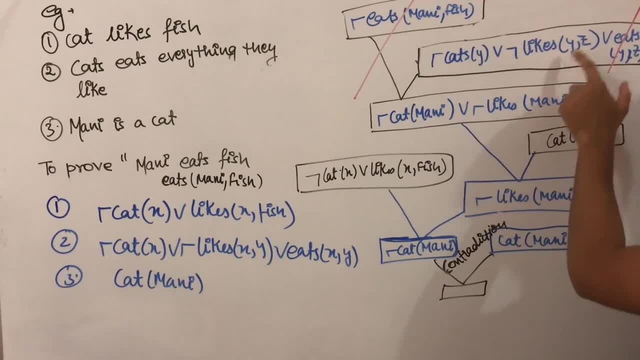 in place, of why you can put the value in place, of why you can put the value money or likes money, comma fish, so from money. or likes money, comma fish, so from money. or likes money, comma fish, so from second statement: now this is remaining second statement. now this is remaining. 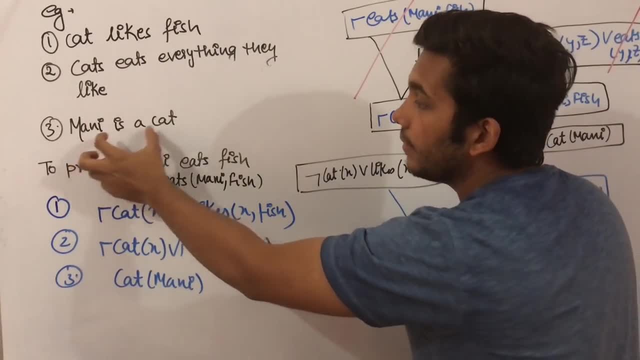 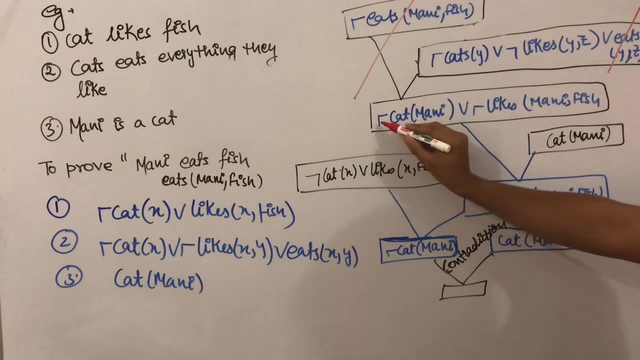 second statement- now this is remaining. and in third statement we have money is, and in third statement we have money is, and in third statement we have money is a cat. so this is our third statement: cat a cat. so this is our third statement: cat a cat. so this is our third statement: cat comma, money. and in this statement we 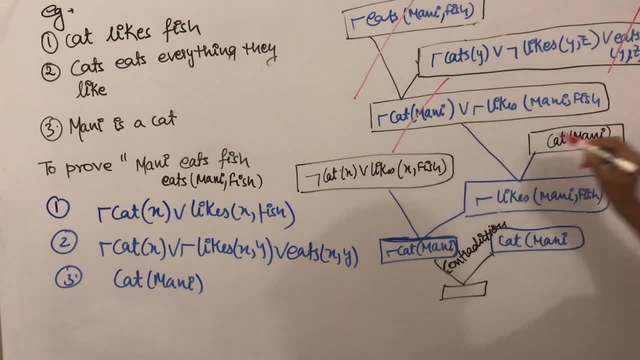 comma money and in this statement we comma money and in this statement we have negotiation of cat comma money. so we have negotiation of cat comma money. so we have negotiation of cat comma money. so we can cancel this part with this part now. can cancel this part with this part now. 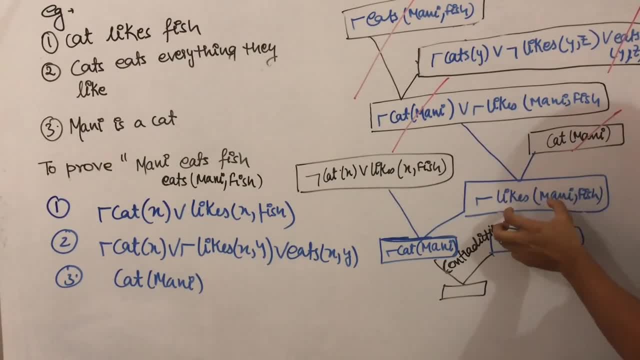 can cancel this part. with this part now, the remaining from this will be. the remaining from this will be. the remaining from this will be: negotiation of likes money comma fish. negotiation of likes money comma fish. negotiation of likes money comma fish. from the first statement we have, from the first statement we have. 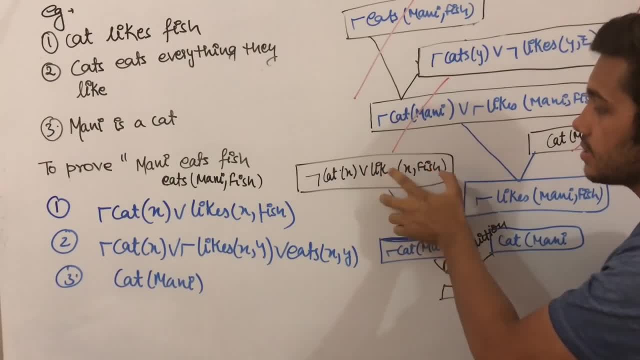 from the first statement. we have negotiation of cat X likes X comma fish. negotiation of cat X likes X comma fish. negotiation of cat X likes X comma fish. and here we have like negotiation of, and here we have like negotiation of, and here we have like negotiation of likes X comma fish. now we will going to 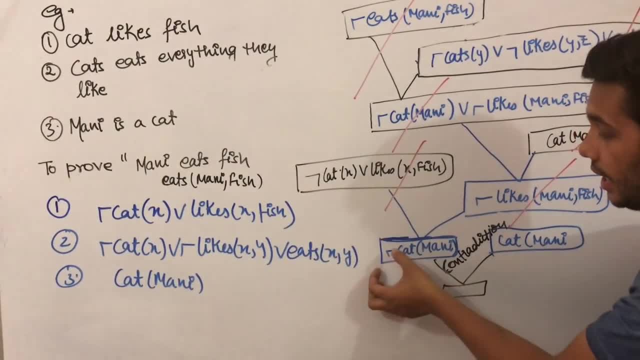 likes X comma fish. now we will going to likes X comma fish. now we will going to cancel this part and this part. and now cancel this part and this part. and now cancel this part and this part. and now remaining will be negotiation of cat money. remaining will be negotiation of cat money. 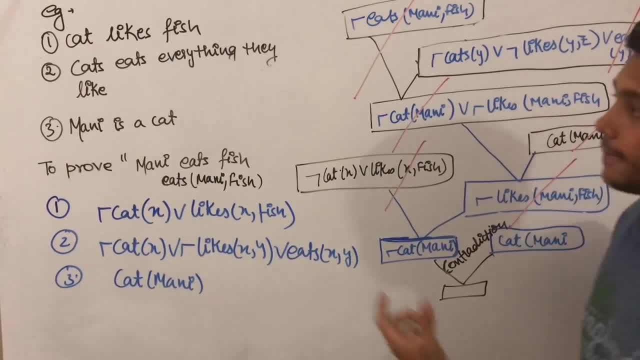 remaining will be negotiation of cat money. this is the remaining okay, but this is the remaining okay, but this is the remaining okay, but in a statement being in a statement, it is in a statement being in a statement. it is in a statement being in a statement. it is given money is a cat. and now what we? 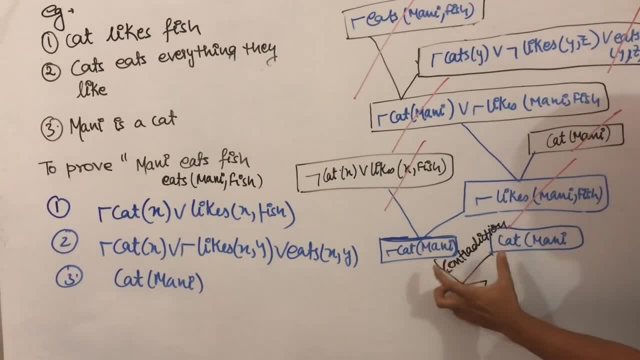 given money is a cat. and now what we given money is a cat. and now what we are getting- negotiation of cat money. so are getting negotiation of cat money. so are getting negotiation of cat money. so what it is, what we have proved, is wrong. what it is, what we have proved, is wrong. 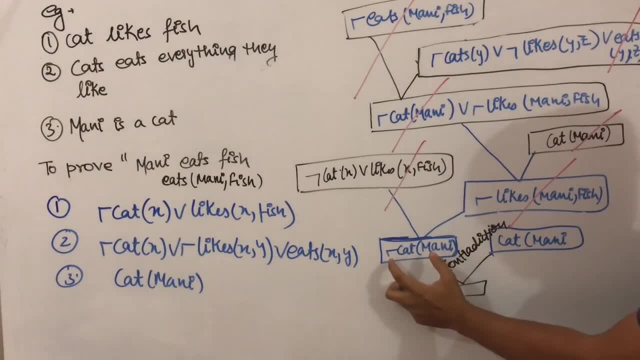 what it is, what we have proved is wrong, so it is approved by contradiction. so it is approved by contradiction. so it is approved by contradiction because negotiation of cat money when. because negotiation of cat money when. because negotiation of cat money when what we have get money. so it is a. 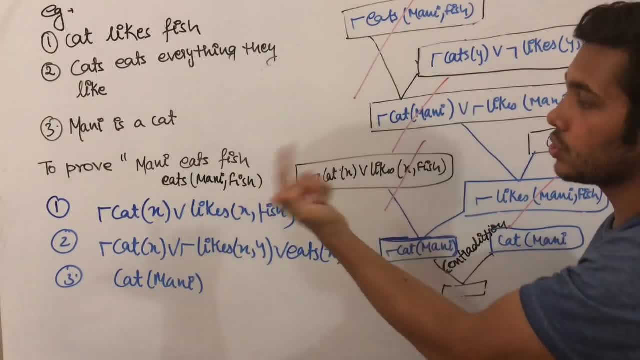 what we have get money, so it is a what we have get money, so it is a contradictory statement. so what we have? contradictory statement. so what we have get money. so it is a what we have get money. so it is a what we have get money, so it is a assume was wrong. so this statement is. 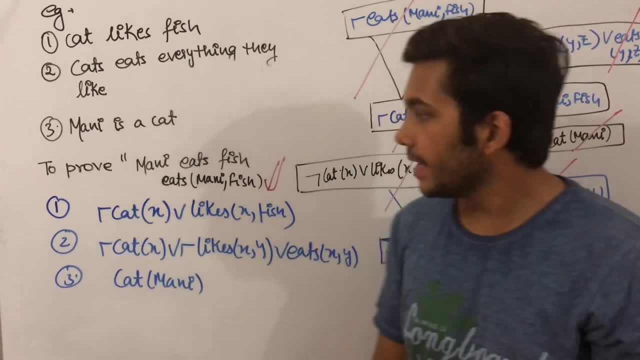 assume was wrong, so this statement is assume was wrong, so this statement is right. so this is how resolution work in right. so this is how resolution work in right. so this is how resolution work in first step. the normal statements are first step. the normal statements are first step. the normal statements are given and from that we need to convert. 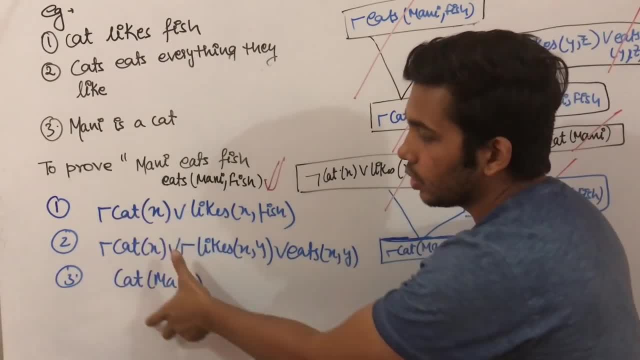 given and from that we need to convert given and from that we need to convert into predicate logic and from predicate into predicate logic and from predicate into predicate logic and from predicate logic we need to convert it into CNF logic. we need to convert it into CNF. 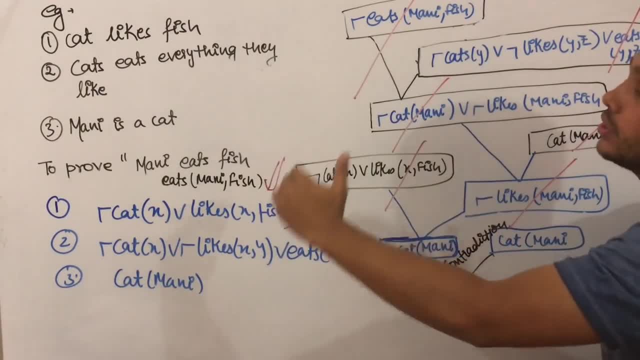 logic. we need to convert it into CNF from and from CNF form. we need to resolve from and from CNF form. we need to resolve from and from CNF form. we need to resolve. each part means, like here the stem what. each part means, like here the stem what. 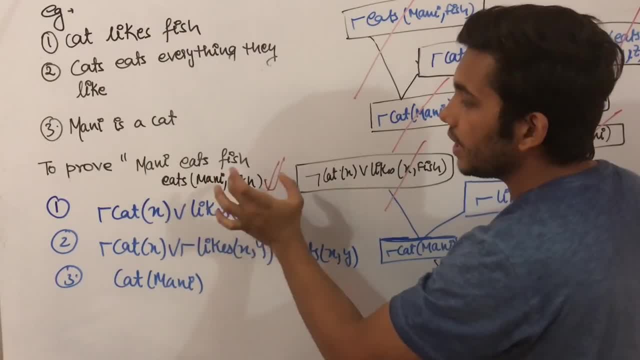 each part means, like here the stem, what we have to prove money each is, we can. we have to prove money each is, we can. we have to prove money each is, we can. write it as each money comma fish, so we write it as each money comma fish, so we. 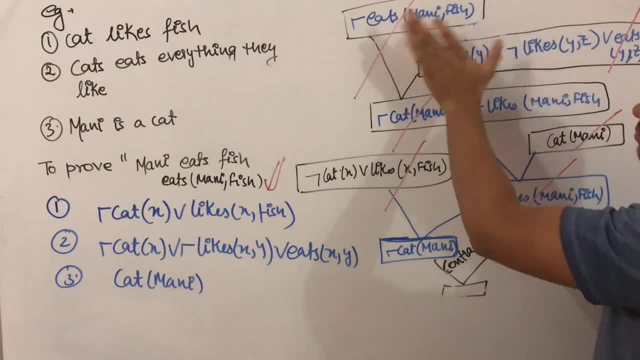 write it as each money comma fish. so we will take the contradictory part. will take the contradictory part. will take the contradictory part. negotiation of each money comma fish and negotiation of each money comma fish. and negotiation of each money comma fish. and from given statements we need to cancel. 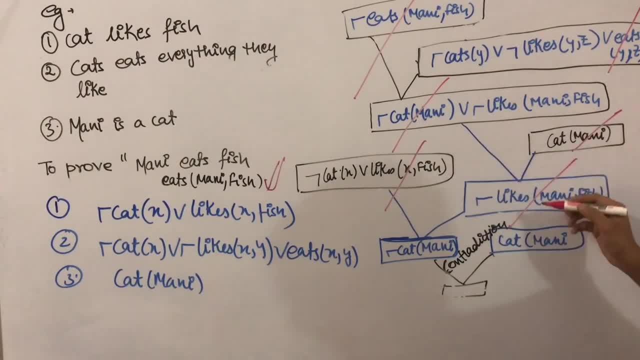 from given statements. we need to cancel from given statements. we need to cancel a positive part with negative part and a positive part with negative part and a positive part with negative part and negative part, positive term and at the negative part positive term and at the negative part positive term and at the end, whatever we will get like. 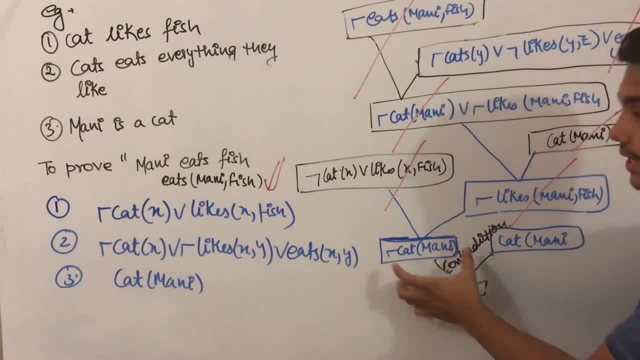 end whatever we will get like. end whatever we will get like. negotiation of cat comma money money. this negotiation of cat comma money money. this negotiation of cat comma money money this weekend. but this is wrong because in weekend. but this is wrong because in weekend. but this is wrong because in the given statement it is money is a cat, so 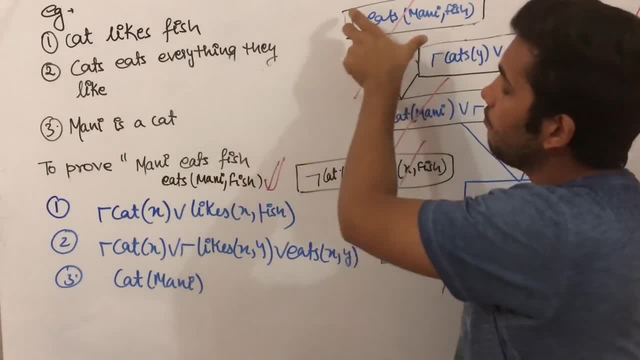 the given statement it is money is a cat. so the given statement it is money is a cat, so it is a contradictory. so whatever we, it is a contradictory. so whatever we, it is a contradictory. so whatever we have assumed was wrong, so money it fish. have assumed was wrong, so money it fish.